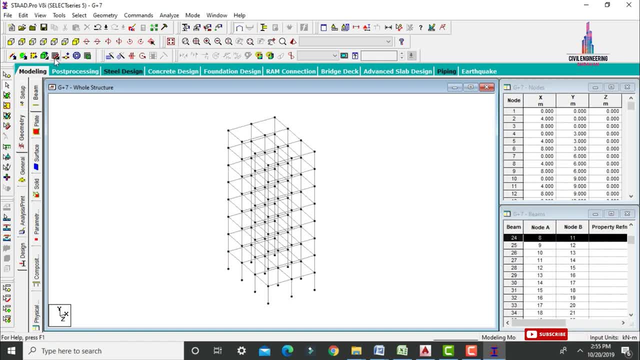 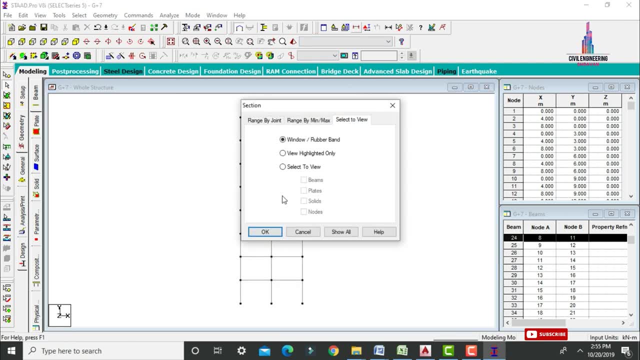 Click on OK. Now we have to import it to the StatPro software here. Now we have to add the staircases for this model. So select the front view. Click on select to view. Click on select to view option. Click on OK. So click on cut this respective ground story. Further select this. 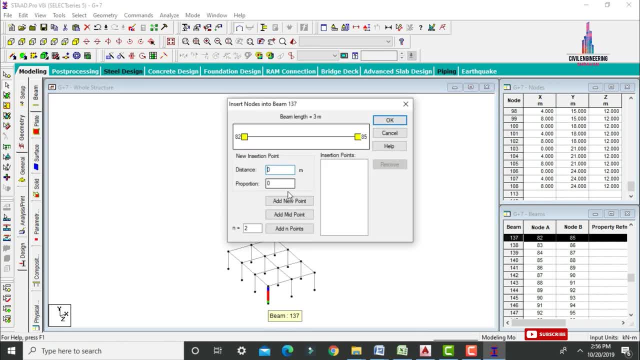 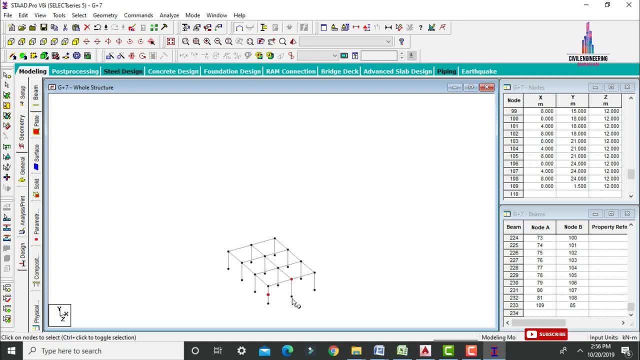 beam. Click on insert a node point at midpoint. Click on OK. Now we have to select the node cursor. Just select the node points here, like this: Just I am selecting the nodes. Click on copy option. Click on paste nodes. Just I am taking Z direction distance. Just I am. 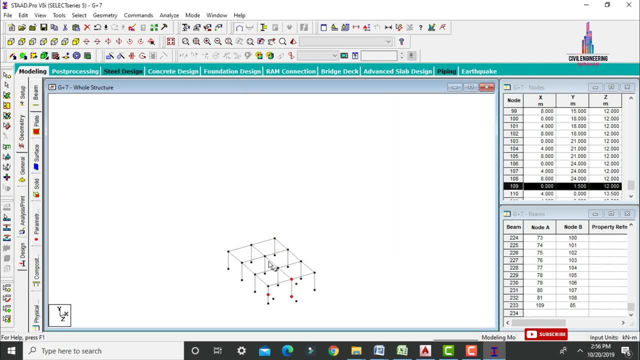 taking winners, which is consisting of one point five meter initially. Again in the same way, again in the same way. click on paste nodes option, which is at a distance of that direction of three meters. So after that we have to select this three node points here. 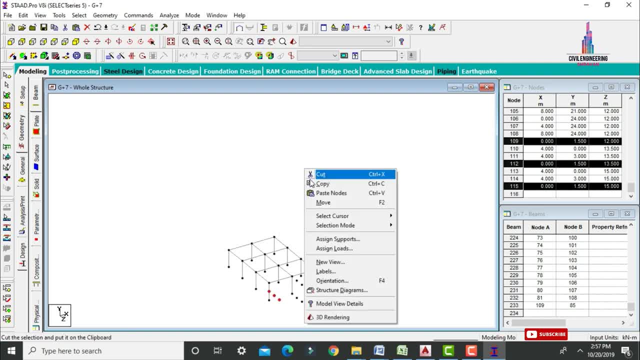 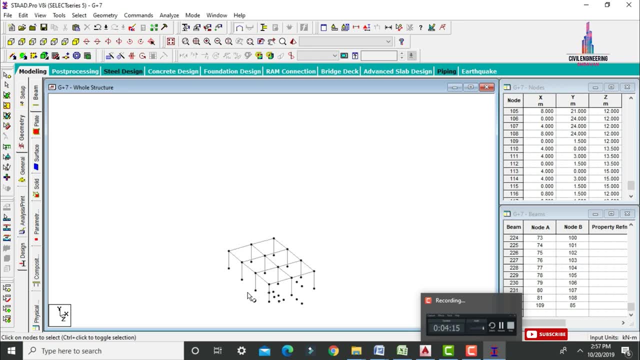 So click on copy option. So here I'm selecting paste nodes which is at a distance of 3.8 Meter in X direction distance. Click on OK. Now we have to connect this node point with the help of SLAM Select. Add four node plate option. select the first point, second, point, three, point four, five. 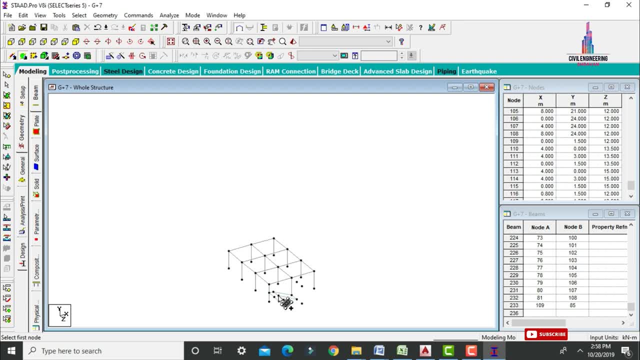 zer gen point. Three points, number of stand, Count them are same, like this Zero point among them: Metic, Perey chi. note this is what we expect to get from Slamp. You can areas. you can add four point. in the same way, we have to connect this respective node points here, like this: now we: 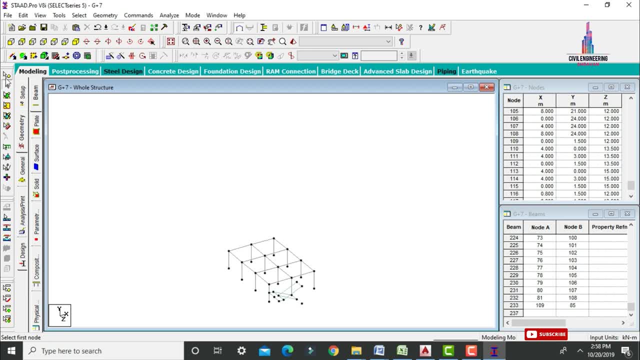 have to connect the cantilever beam here. select add beam command, select the first point, select the second point. so in the same way we have to copy this cantilever beam to the x direction distance which is consisting of 4 meter. so click on copy option, again click on paste beams which 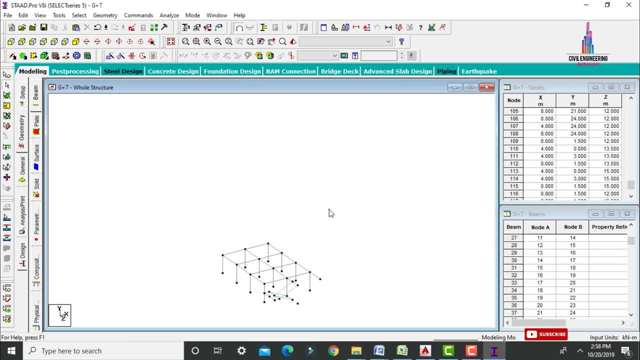 is at a distance of x direction distance of 4 meter. so after that we have to create the uh slab section for the ground story. initially select, add four node plate select: first point, second point, third point, fourth point. so in the same way, just i'm adding the slab section for the 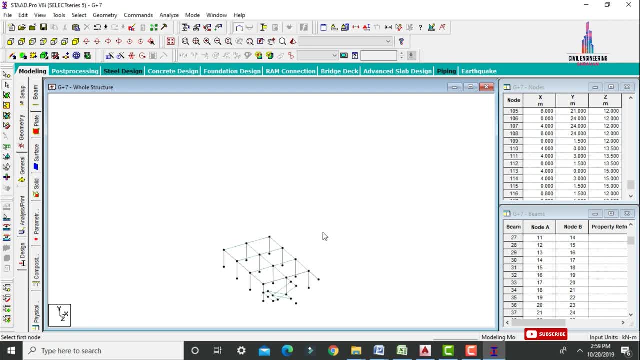 remaining building. so after that click on whole structure command here. now we have to copy the slab section from the ground story section to the remaining three stories. so for that, initially we have to select the slab cursor here. so select the slab cursor. select all the slabs, so go to. 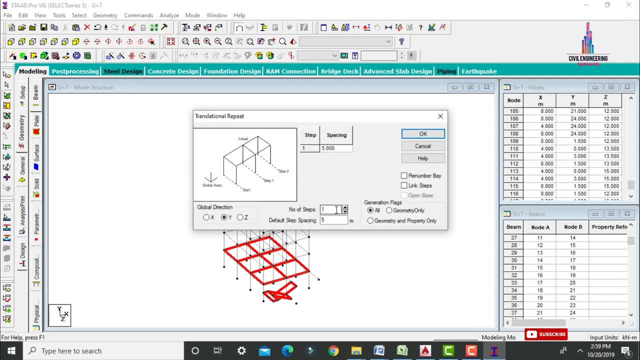 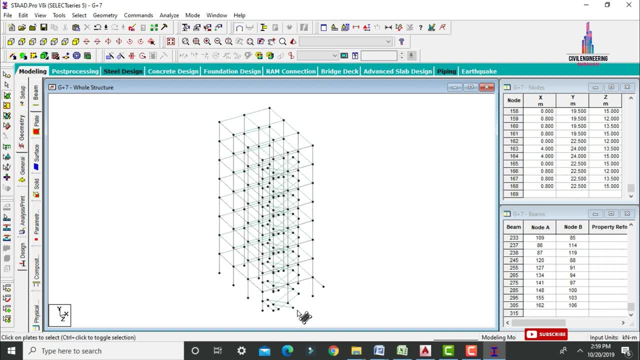 transitional repeat option in y direction. number of steps will be consisting of seven and each step will be consisting of three meter. click on ok. now it was copied your respective slab section here, so after that we have to copy the beam sections here. select these respected beams. go to transitional repeat in y direction number. 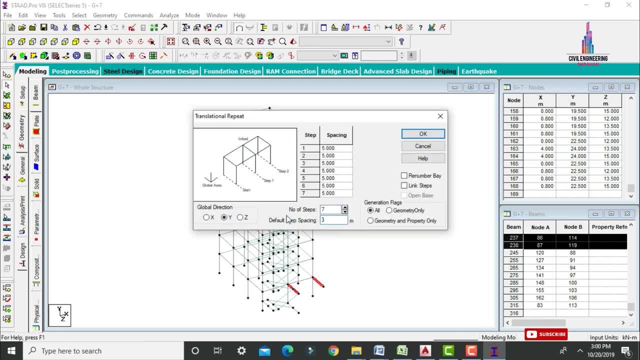 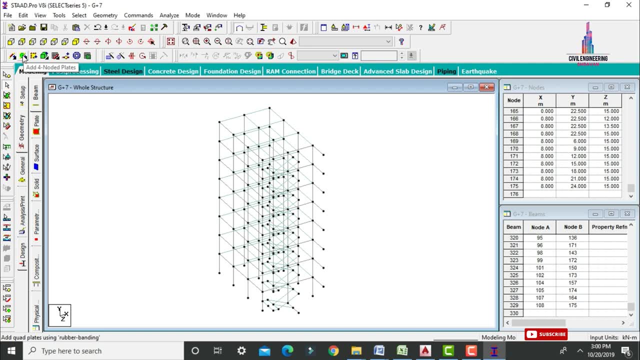 of steps will be consisting of seven and each step will be consisting of three meter. click on ok so it will copy your all beams here like this: now we have to connect the uh respected cantilever slab with uh add four node plate option. so select first point, second point, third point, four. 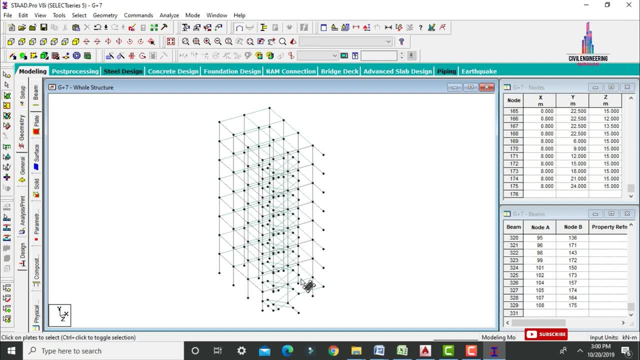 point. so after that, select the uh plate cursor. select this slab, go to transitional. repeat in y direction. number of steps are seven and each step will be consisting of three meter, so after that we have to apply the properties for this building. call to click on general option. select the. 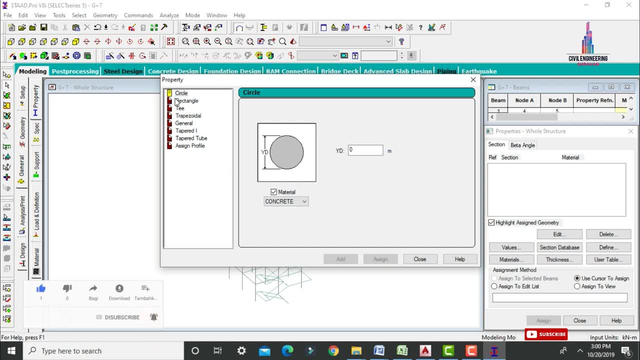 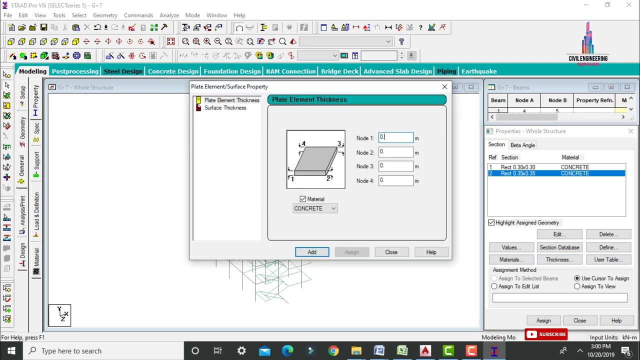 property. click on define. just i am taking the rectangular section which is consisting of 0.3 cross 0.3 is the beam size. again i am adding the rectangular section which is consisting of 0.35 cross 0.35 column size. so click on thickness option, this time giving the slab thickness which is consisting of: 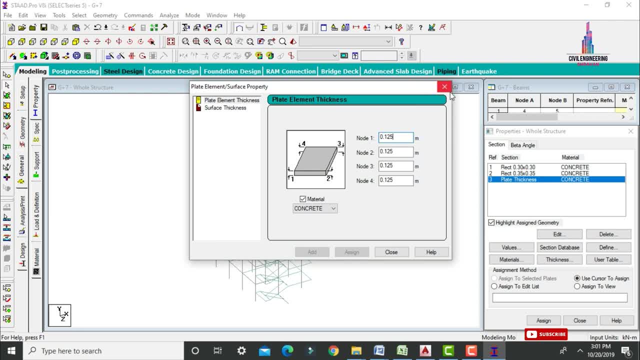 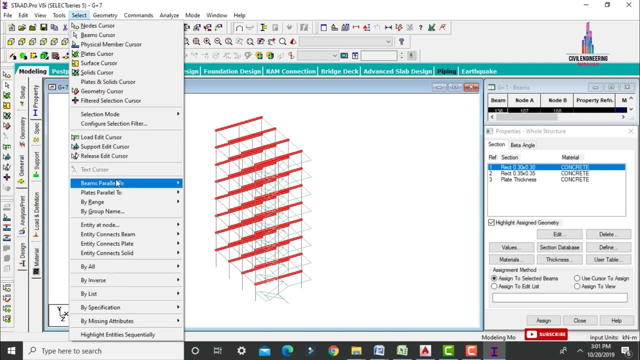 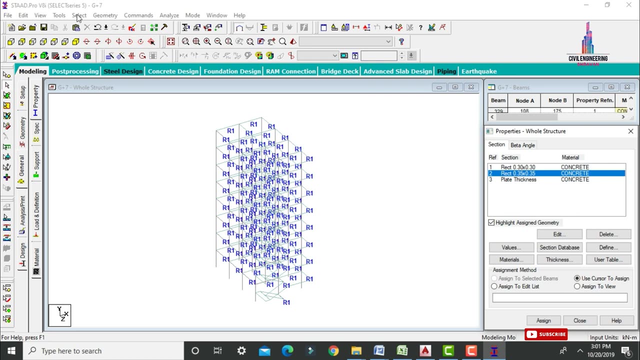 125 mm. now we have to assign this properties for the building. select 0.3- 0.3. we have to select the beams parallel to x condition. again i'm selecting beams parallel to z condition. click on assign to selected beams. assign yes option. now i'm selecting 0.35, cross 0.35. we have to select beams parallel. 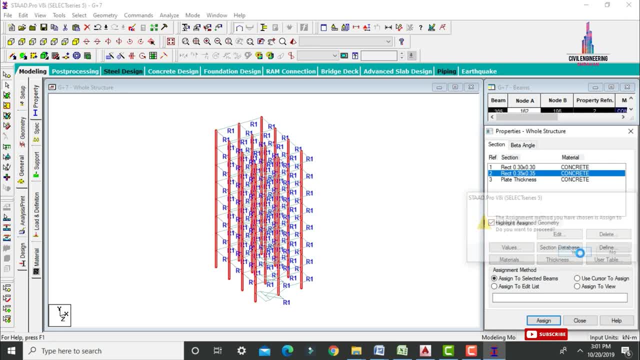 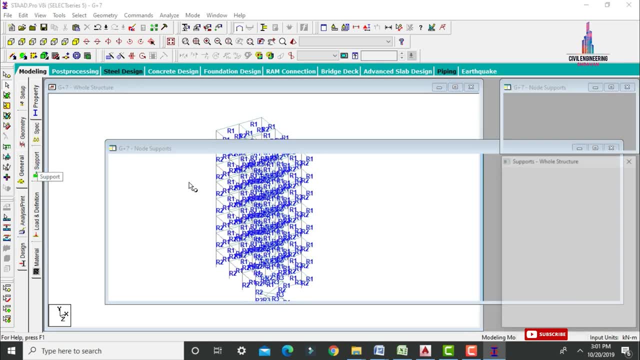 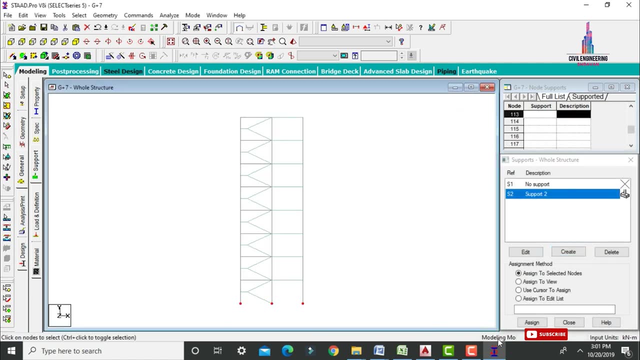 to y condition. click on assign to selected beams. assign yes. now i'm selecting plate thickness by using assign to view assign yes option. so after that we have to assign a support. select the supports option. click on create add your fixed support. select your support to. so we have to select all the node points at the base. click on assign to selected nodes: assign. 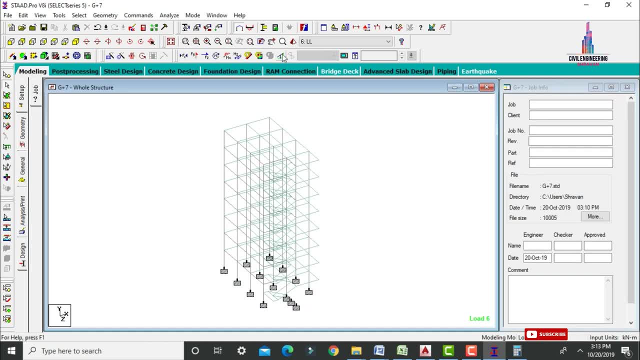 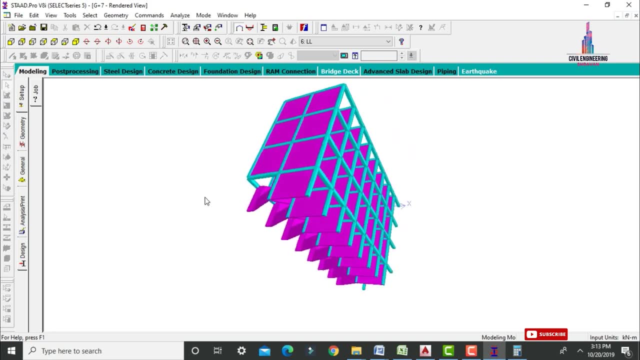 yes option. so after that, click on 3d view. so this is the 3d rendering view for this respected building. it will be consisting of 0.35 cross 0.35 is the column size and 0.3 cross 0.3 is the beam. 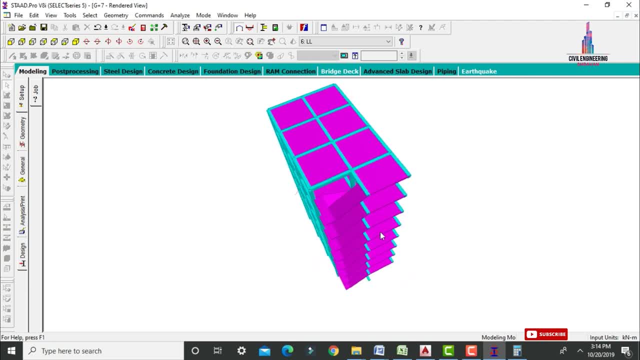 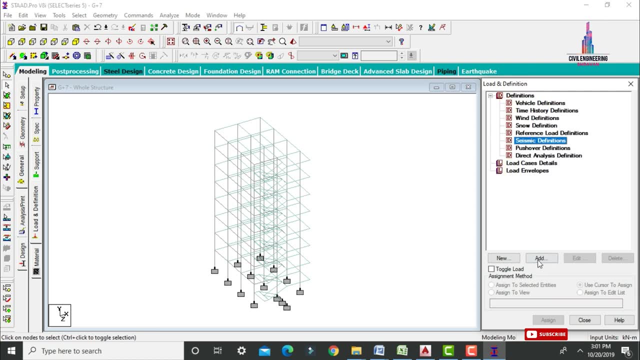 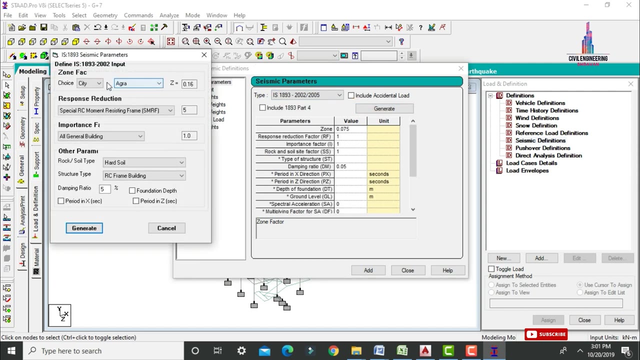 size and slab thickness will be consisting of 125 mm. so after that we have to apply the load cases. click on definition: here initially i'm selecting the seismic definition. click on add option. so here we have to select the is code. so click on generate option. now, here we have to select the high seismic zoning condition, which is nothing. 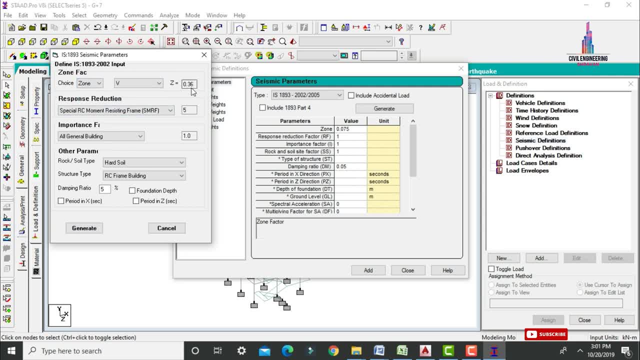 but zone 5 condition, so which is having factor of 0.36. again, in the same way we have to select the response reduction factor. so the response reduction factor, just i'm considering it as special rc movement resisting frame and importance factor as one which is in a loose soil condition. 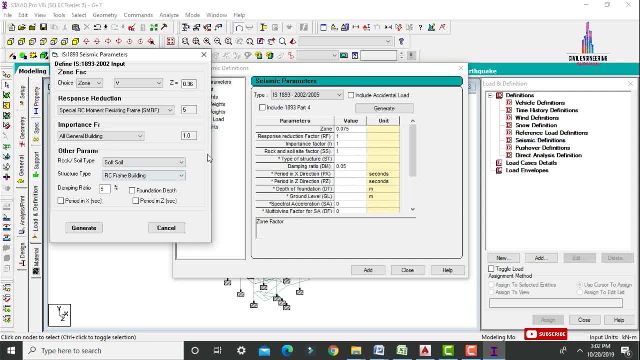 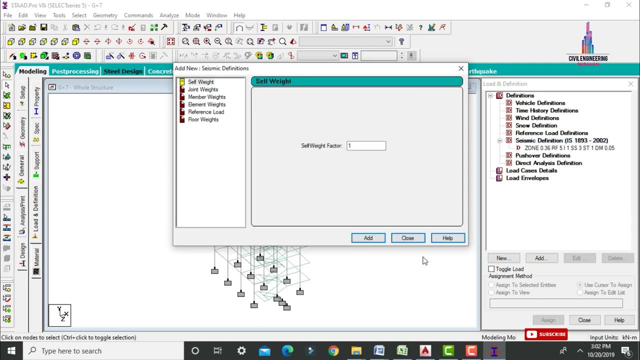 okay, just i'm considering varistic is here, which is in loose soil condition, so after that we have to select the rc frame resisting building. just i'm considering this damping ratio as 5. click on generate option. again we have to change this respected value to 0.05. click on add. now we have 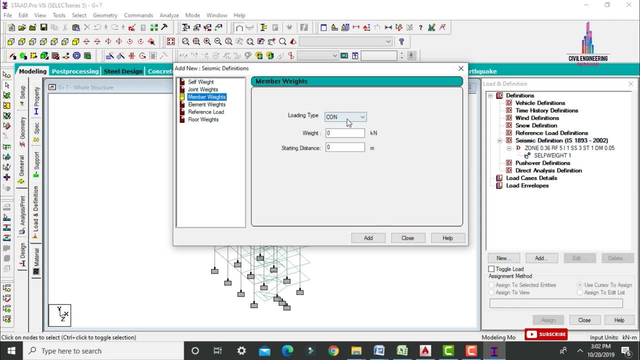 to add the self-heat as one. again i'm adding member weight which is consisting of uniform load. so we have to add the self-heat as one. again i'm adding member weight which is consisting of uniform load. so here we have to calculate the intensity of the beam dead load. so depending upon 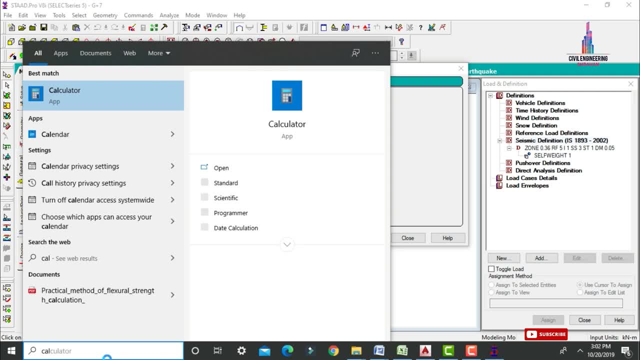 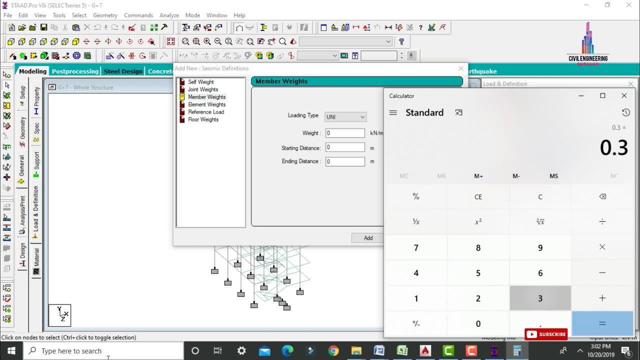 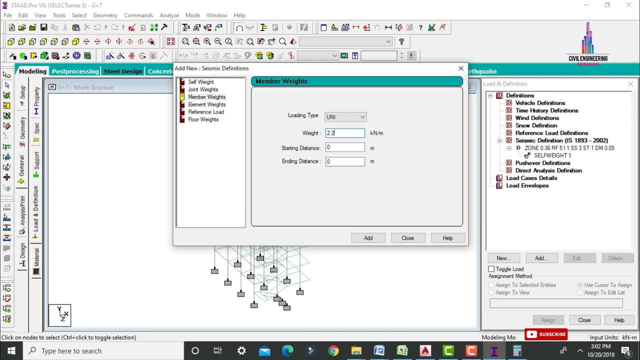 the beam dead load, the value of your respected or 0.36 will be varying. okay, so here i'm considering 0.3 cross 0.3 is the dimensions of the beam. we have to multiply this respected value with 25 so it will give the intensity of 2.25- 2.25. click on add option. close option. select 2.25. 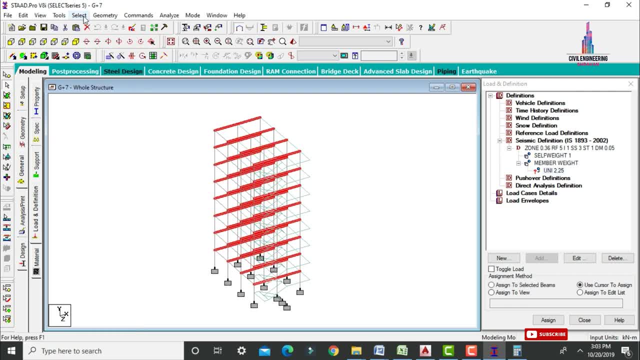 we have to select the beams parallel to x condition. again we have to select the beam parallel to z condition. click on assign to selected beams option. assign yes option. so after that we have to define the wind loading condition. select wind definitions, add button. now we have to select: 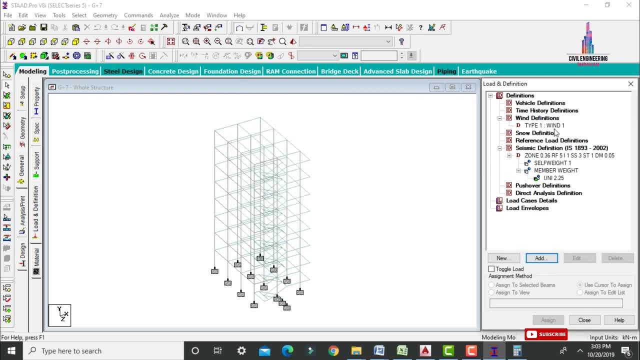 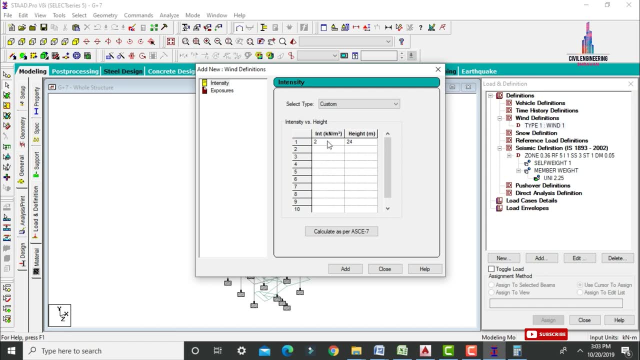 type 1 window. add- close. select type 1 window on here. so click on add option here. so here i'm taking the intensity as 2, which is acting at a distance of 24 meter. again i'm taking one more intensity, 1.5, which is acting at a distance of 18. again i'm taking one intensity which is acting at a distance. 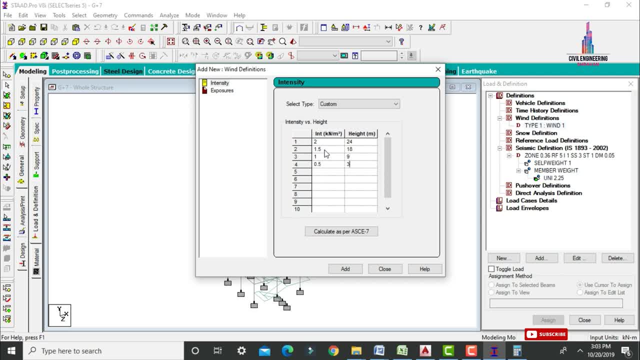 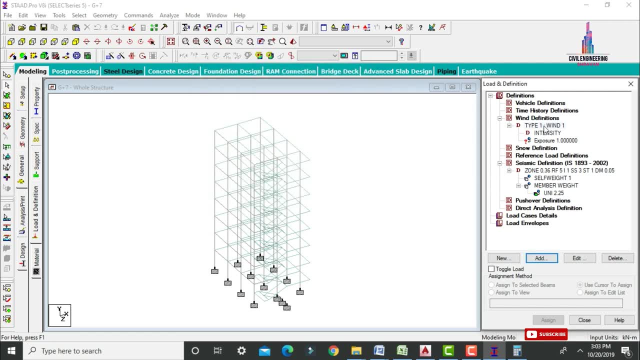 of 3.. again, i'm taking 0.5, which is acting at a distance of 3.. click on add option. so after that we have to take the exposure factor as 1. add button. close option. now i'm selecting exposure 1. click on assign to view assign yes option. so after that we have to select the load case details add. 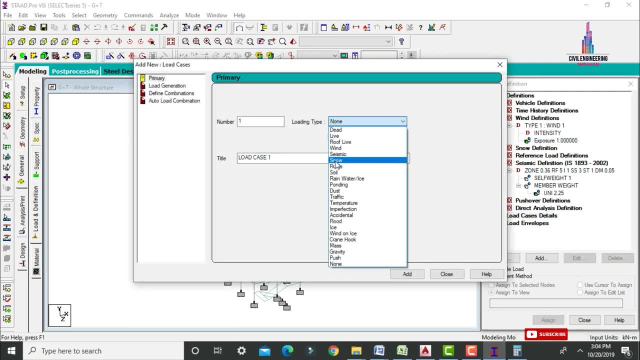 button. initially i'm selecting the seismic loading condition, which is in x direction condition, earthquake load x. again i'm selecting earthquake load in z direction condition. so in the same way i'm taking these two loads, i am selecting the load title as l, l and i have 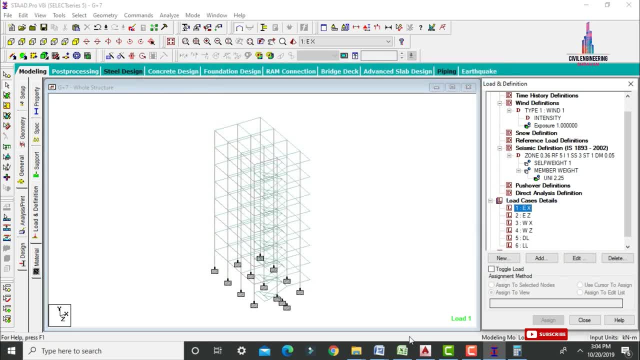 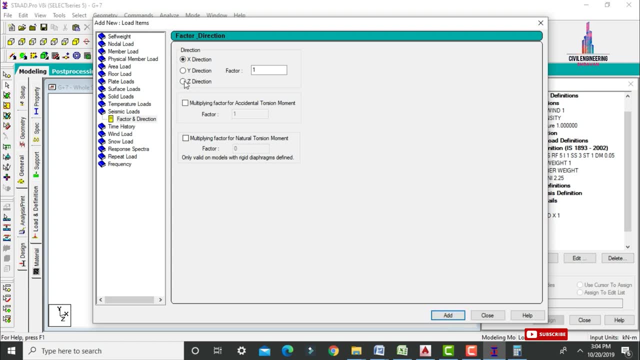 to take the static load section. now i'm selecting earthquake load and drag on alerts direction. scene icon is ஆn in the background. click on add so select the seismic load. similarly, click on add. pinned on lane in z direction. click on add. select the seismic load which is in z direction with the factor one. 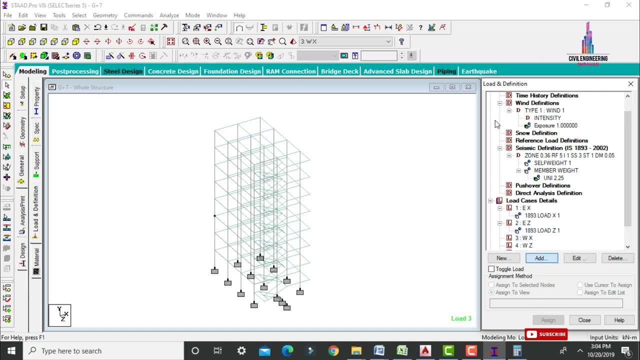 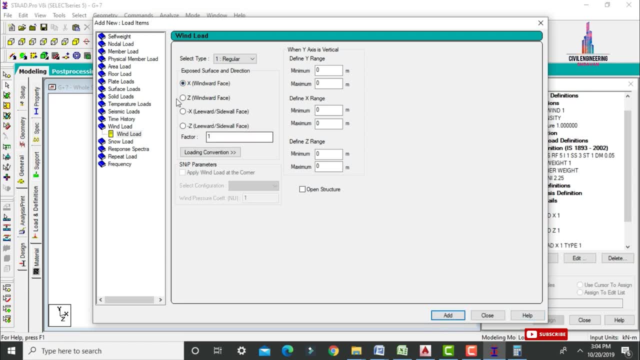 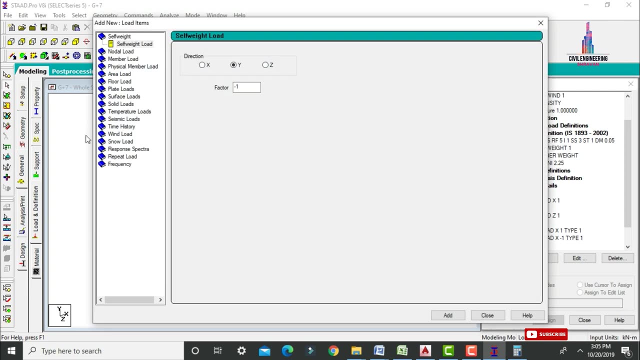 and close. select windex add button. so here i'm selecting the load case as wind load which is in x direction with the factor one add button. again i'm selecting minus one factor. so after that we have to select the wind load in z add option. now i'm selecting wind load which is in z condition. 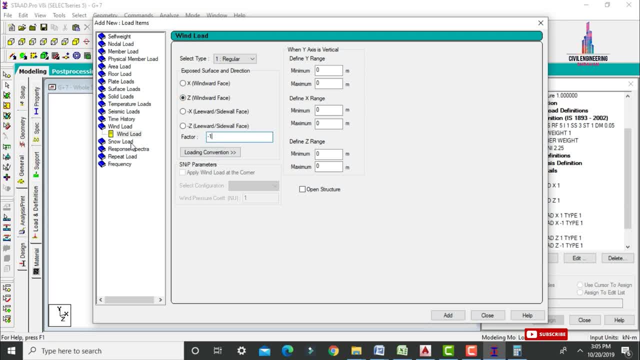 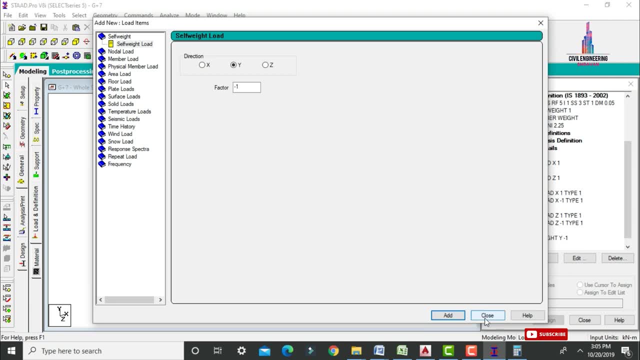 with one factor. again i'm selecting minus one factor. now in the same way. just i'm selecting gate load condition. click on select. add your self-aid here. so select self-aid by using assign to view, assign, yes option. now i'm selecting live load by using add button. we have to select the 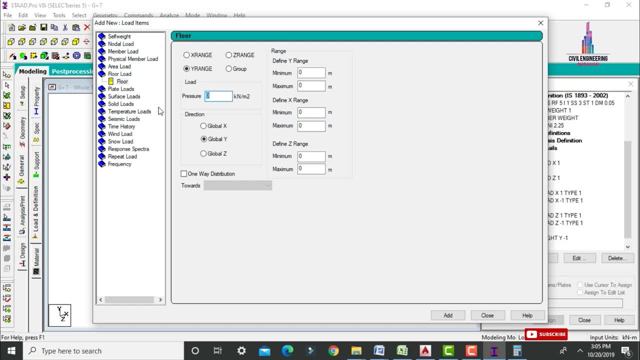 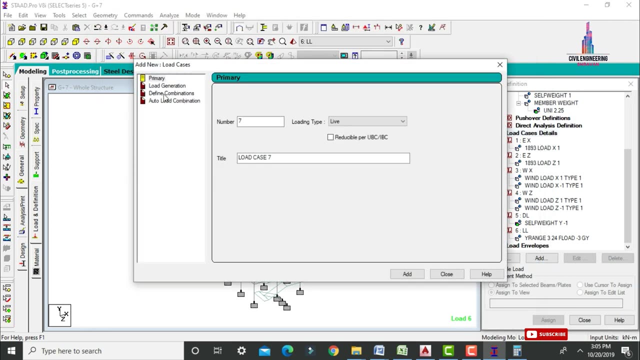 floor load which is consisting of just- i'm assuming it has- minus three, which is acting at a distance of three meter and 24 meter. click on add button- close option. so after that we have to add the load count here. select load case details. click on add button. select auto load combinations option. select it. 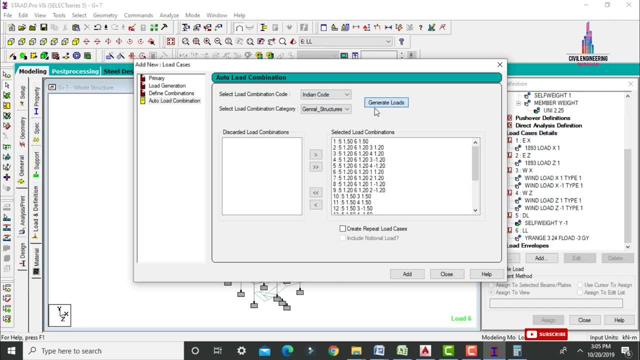 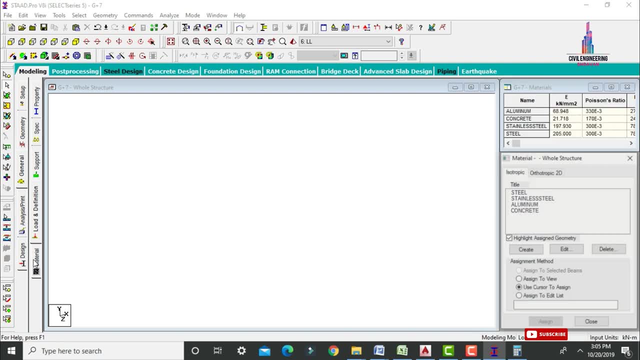 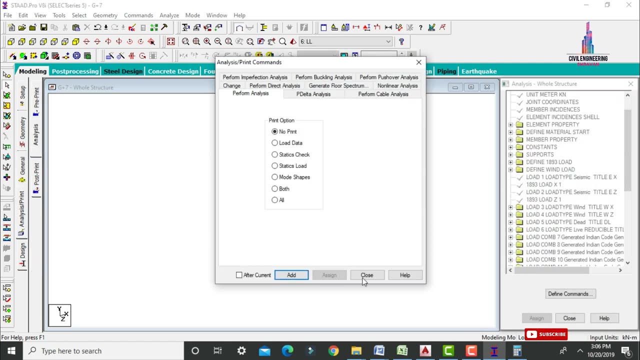 as indian standard system. click on generate so it will generate the load combinations as per indian code. click on add button- close option. now we have to go to materials. click on concrete assign to view. assign yes option. now i'm selecting analysis and print. add your no print- close option. 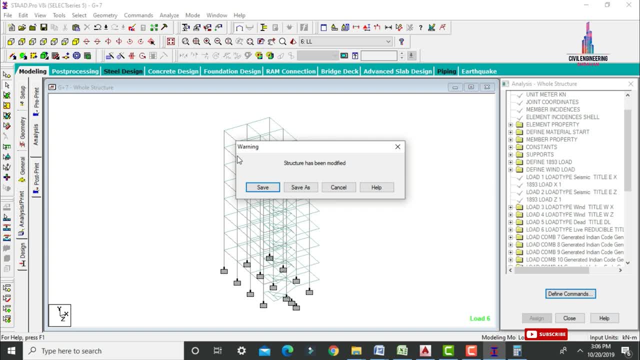 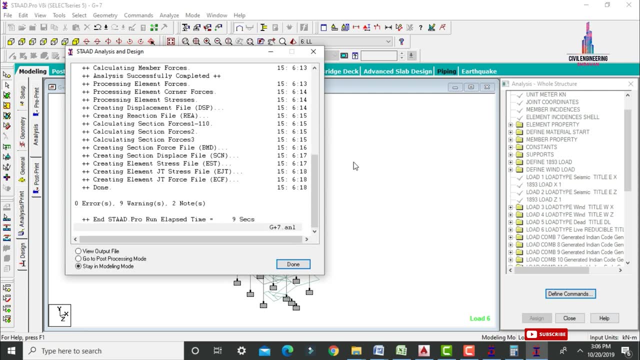 go to analyze option: run analysis, save it. so here we have to check for the zero errors for this model. so here my model is checking for the zero errors. so here my model is observed with zero errors. go to post processing mode. click on done option. so click on apply, click on okay, so 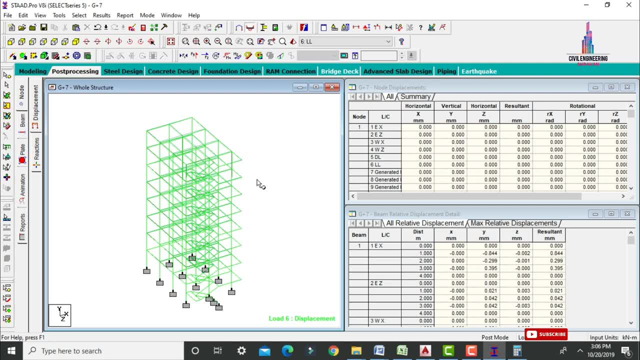 this is the deflection of the building due to presence of the live loading condition. so here i'm taking earthquake load in x direction condition. so initially i will show you the deflection in front view. due to presence of the earthquake load in x direction, the deflection of the building is more. 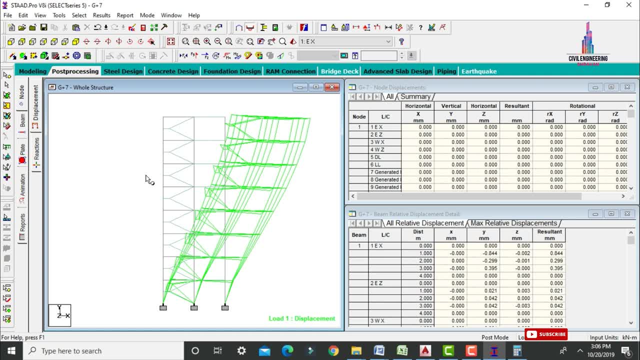 why? because we are taking the parameters which is related to the high seismic zoning condition and loose soil condition. due to this two parameters, the building is deflecting like this. okay, so after that we have to select the earthquake load z, again side view. so this is the deflection due. 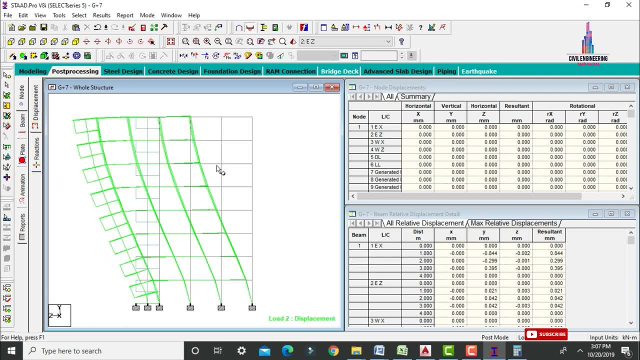 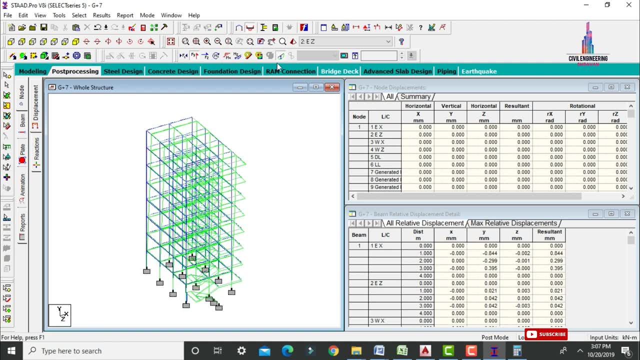 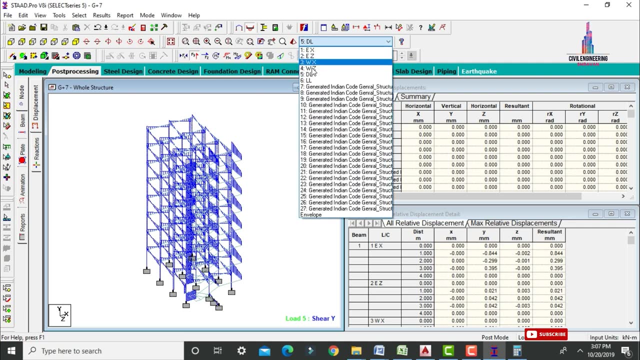 to presence of the earthquake: loading z direction condition. now we have to check the shear force diagram, bending movement diagram. so select fy. so this is the shear force diagram for this building. due to presence of the growth in y direction condition: select the dead loading condition. select the live loading condition. again i am selecting mz work. 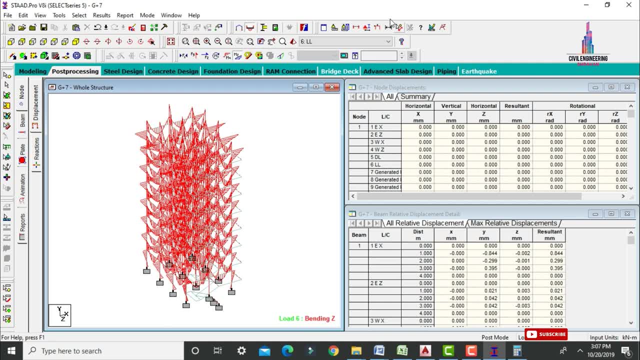 So this is the bending moment diagram for this respected model, due to presence of the earthquake load x. earthquake load z. wind load x. wind load z dead load, live load condition. So after that we have to check the plate load, select the plate load, select stress type as: 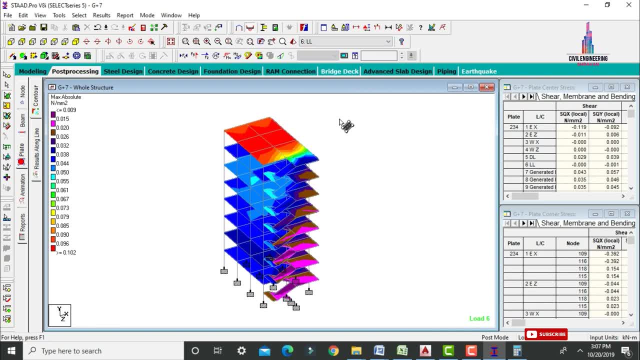 absolute pressure: apply okay. So this is the absolute pressure for this building due to presence of the various types of load cases. So after that, go to select animation. click on deflection. click on apply. click on OK. So this is the deflection of the building due to presence of earthquake. compon Galaxy. 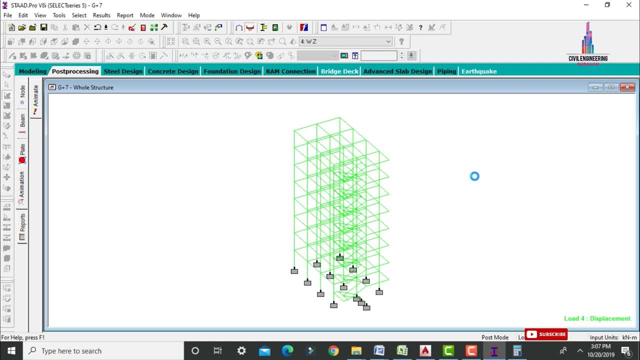 3: x direction: earthquake, Z Direction condition: wind x, wind y, dead load conditions, live load conditions. So, after the analysis process completed, we have to design this building. So, due to presence of the earthquake loading X direction condition which is in high seismic, 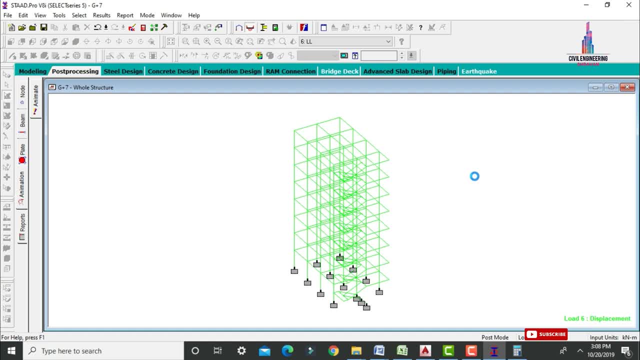 Zoning condition and earthquake loading Z Direction condition in is nationalism. in terrain Zoning condition, We are concluded that the building deflection value is higher in case of the seismic loading condition. then remaining load cases. Okay, so after that, click on modeling option, click on design, click on concrete design. so here, 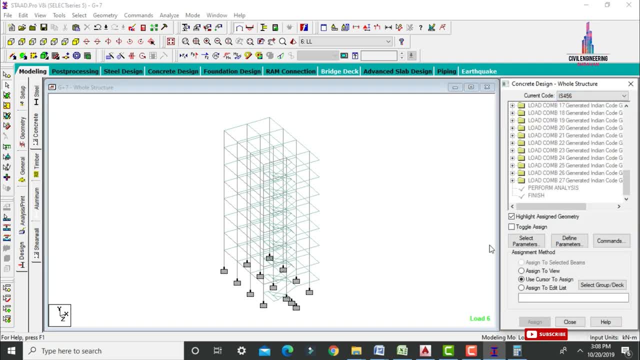 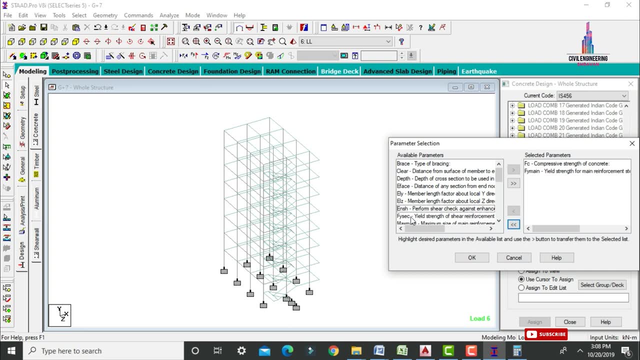 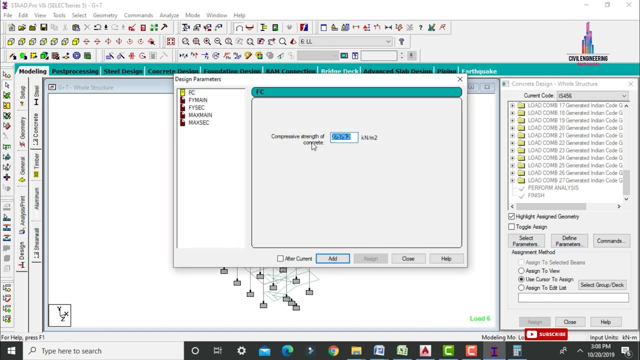 i am selecting as per the indian standard system. click on select parameters. initially we have to deselect all parameters. select the compressive strength yield, strength yield, strength of shear reinforcement maximum and maximum secondary. click on ok option, select, define parameters. so here i am considering m30 grade concrete for designing of this respected. 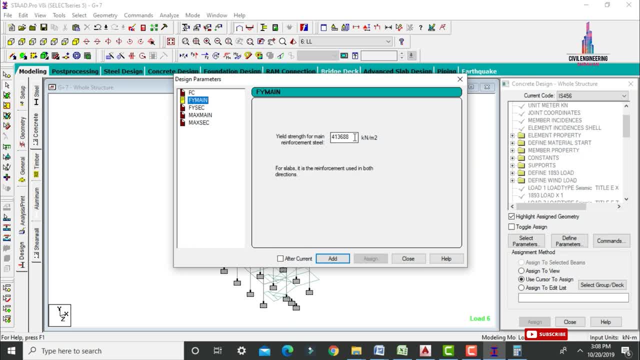 building: again i am taking fe 500 grid steel: 500 000 click on add button. again i am selecting fi section, also 500 000 click on add button. again i'm selecting maximum main: just i'm taking it as 20 m. again i'm selecting maximum secondary: just i'm taking it as 16 m. add button. close option. 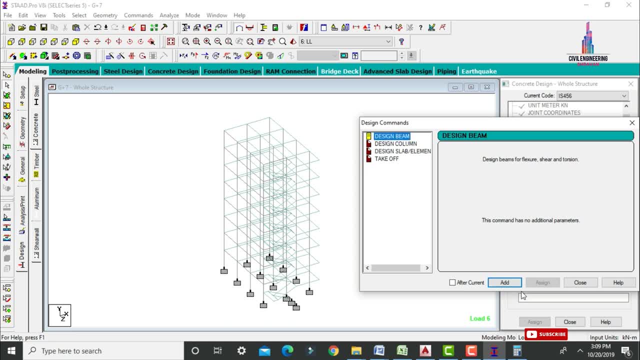 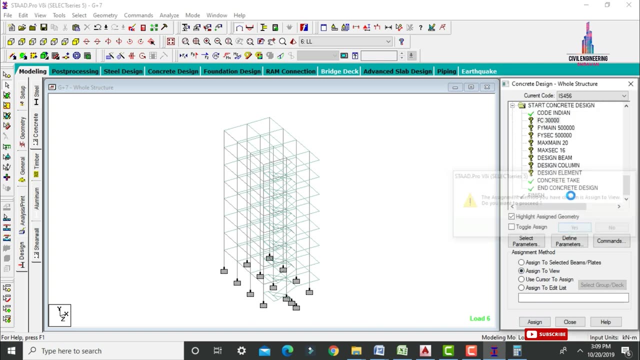 select the commands here: click on: select design beam: add button. select design column: add button designs. labelman command: add button. take off command- add button- close option. after that we have to select the quotient marks here: select fc by using: assign to view. assign yes option by using fy: assign to view. assign yes option. again i'm selecting fi section: assign to view. 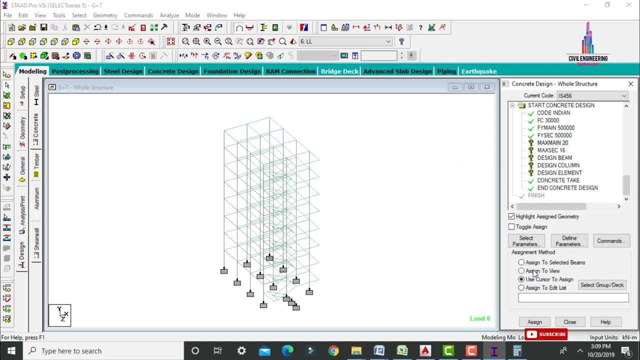 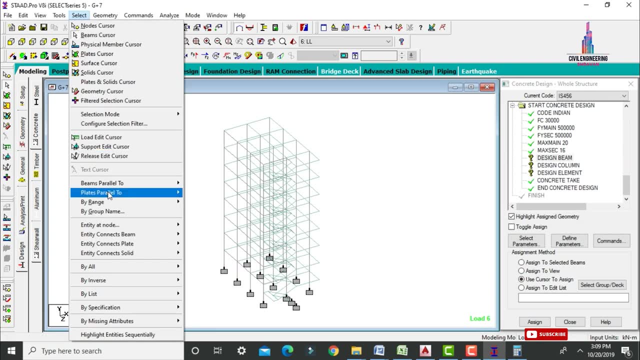 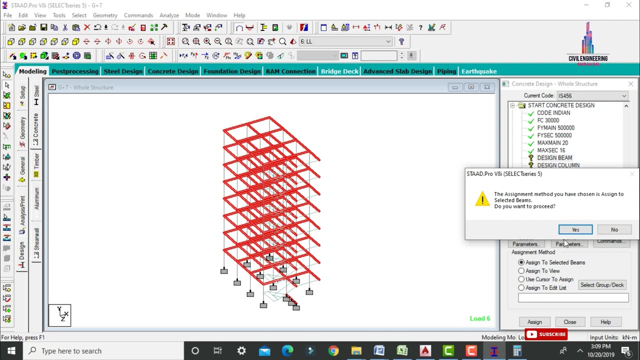 assign yes option: maximum main. assign to view. assign yes option: maximum secondary. assign to view. assign yes option. click on design beam. we have to select the beams parallel to x condition. i have to select the beams parallel to z condition because sent to selected beams. assign yes. select design column. 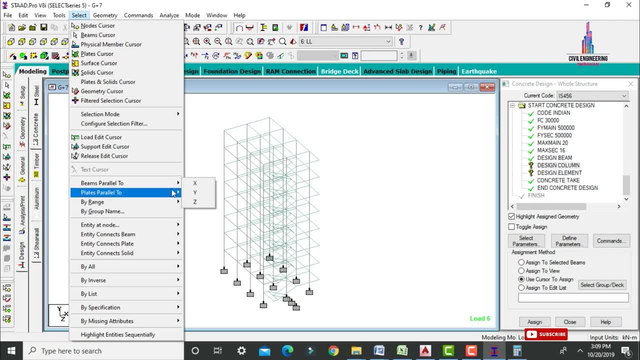 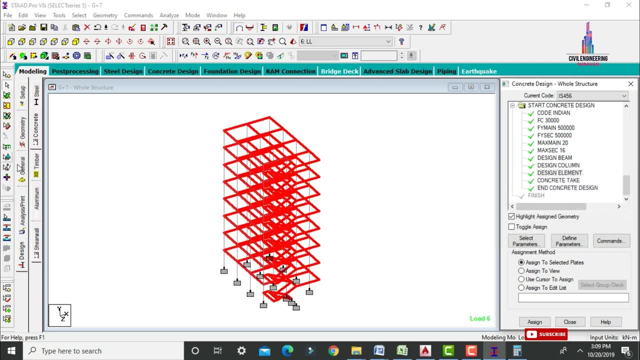 go to select beams parallel to y axis. click on assign to selected beams. assign yes. select design element. assign to view: assign yes option. now we have to go to analysis and print. add your no print close option. again go to analyze option. run analysis, save it. so here we have to check for. 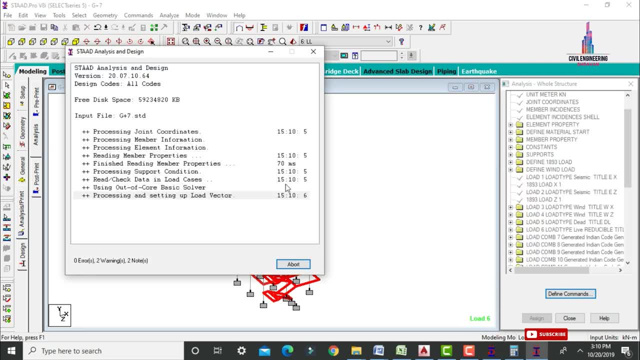 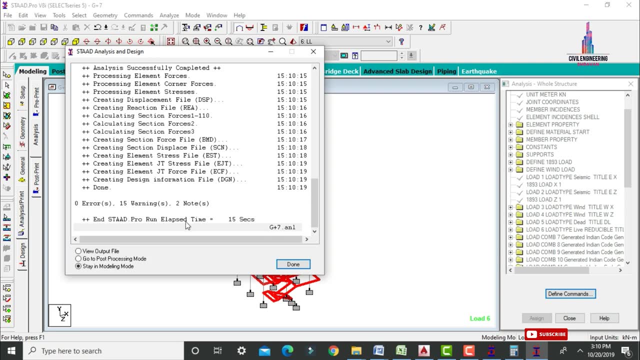 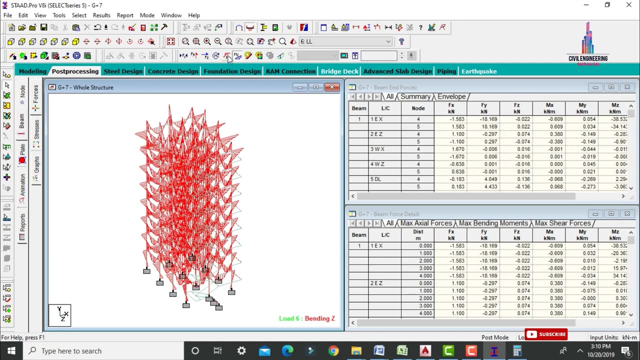 the zero errors for this respected model also. so here my model is checking for the zero errors. so here my model is observed with zero errors. go to post processing mode. click on done option. so we have to click on beam option. so deselect that. bending my diagram, select any one of the beam here. 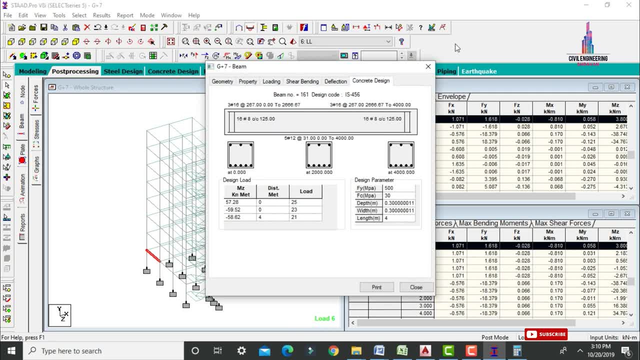 just double click on it. click on concrete design. so, due to presence of the high seismic zoning condition for designing of this respected building of uh, having beam number of 161, it was required three bars of 16 mm at the top reinforcement section and five bars of 12 mm at the bottom. 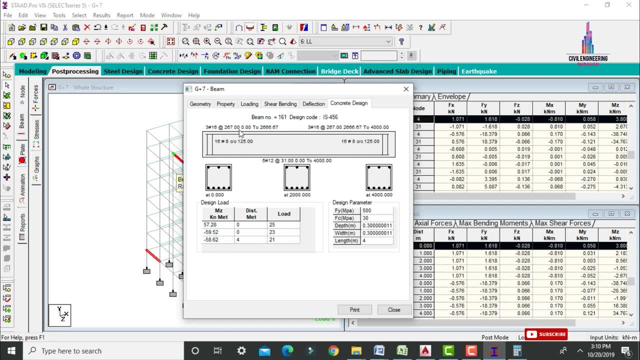 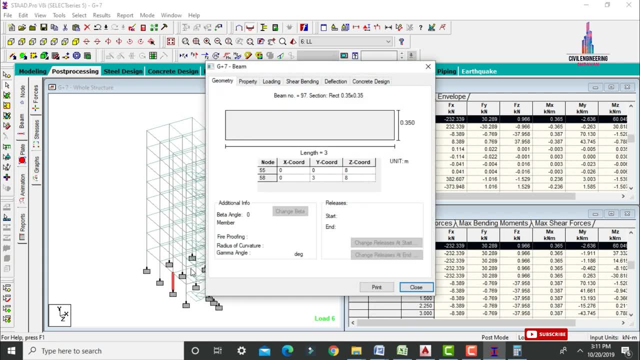 reinforcement section, okay, which is having center to center distance is 267 meter, so 267 mm. so after that, select any one of the column. just time selecting column, double click on it. so click on concrete design. so this is the concrete design for this respected column. it will be consisting of: 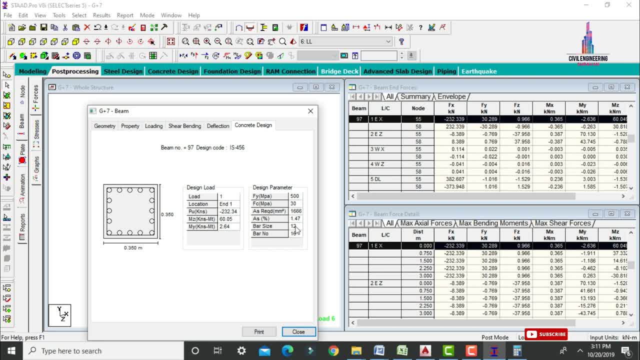 16 number of bars of 12 mm dia. so for construction of this respected building it is required 16 bars, which is having 12 mm dia and hd percentage is 1.45 and hd requirement is 1: 6 mm square, which is related to the m30 grade concrete, fe 500 grade steel. so after that we have to check the output. 5. 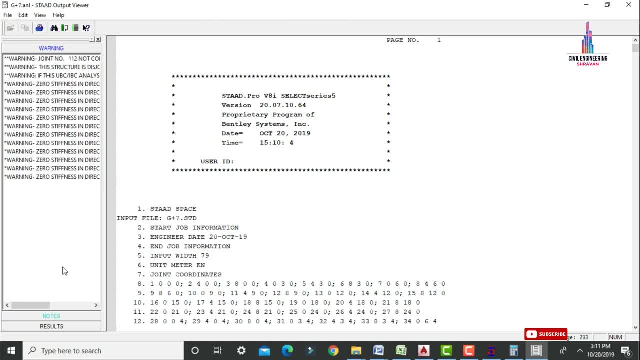 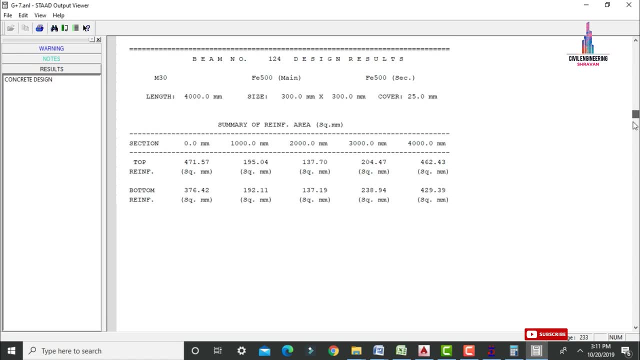 so click on start output file option. so click on results option. click on concrete design. so this is the concrete design values and each and individual calculation part for designing of the building which is in high seismic zoning condition. so after that we have to design the foundation. click. 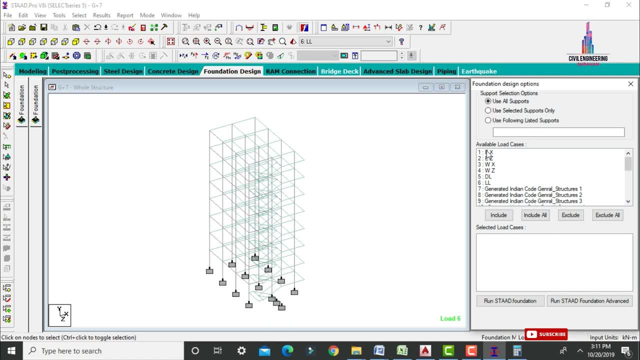 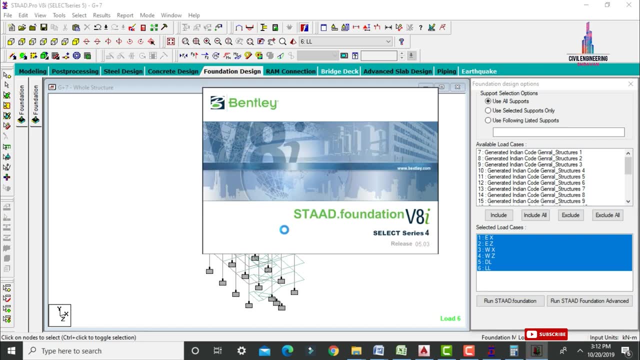 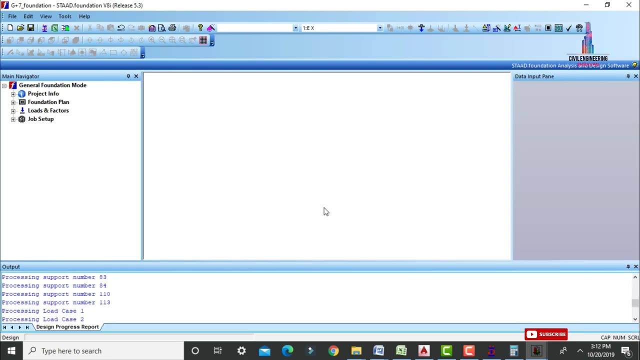 on foundation design. so here we have to select: earthquake load x. earthquake load z. wind x. wind z. dead load, light ink load. click on run stat foundation. the fixed supports of this respected high seismic zone building will be directly imported to the stat foundation software. so these are the fixed supports. we have to design the foundation for this. 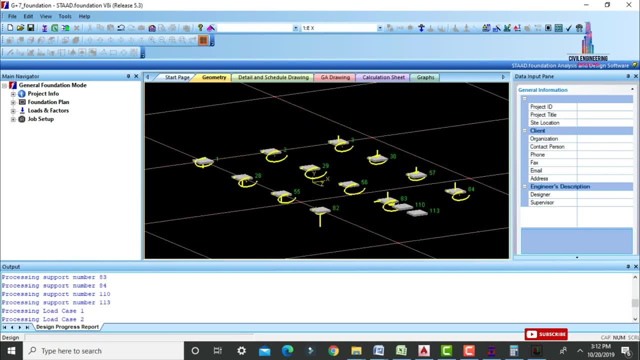 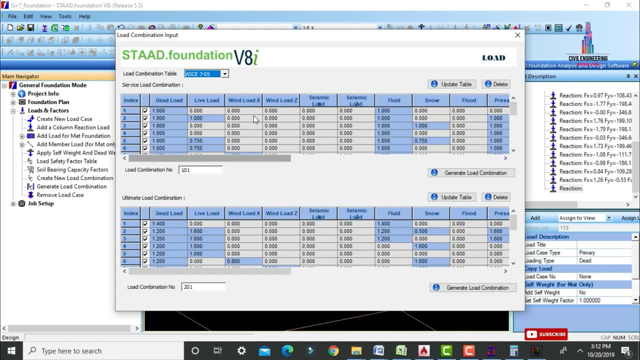 fixed supports only. so initially we have to generate the load, loads and factors. so here i am selecting generate load combinations. so select as per the indian standard system. click on generate. again i am selecting as per the ultimate load combinations. also click on generate, click on ok. so after that cancel this. click on job setup. create job. e the job. 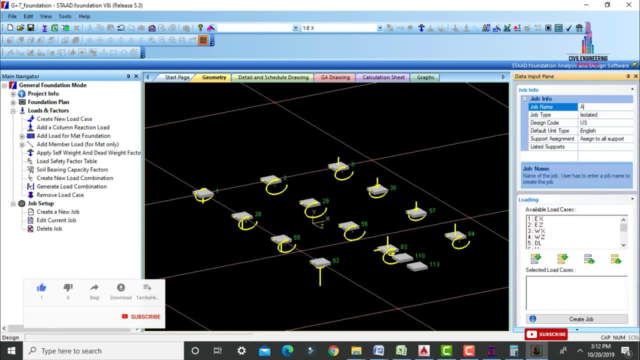 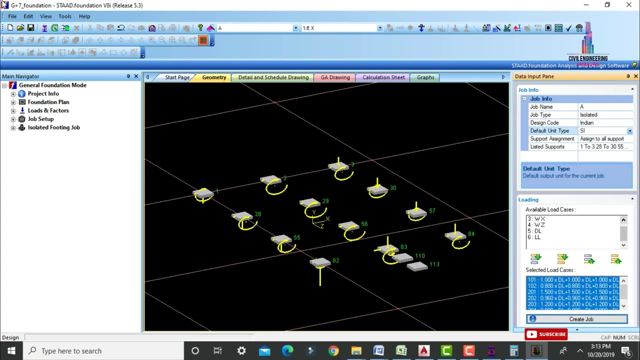 name. just i am taking it as a isolated footing which is having as per the indian standard system and units will be in SI. so here i am including the load cases which is related to the load combinations. click on include. click on create job. so it will create the isolated footing job here like this: select the place mark. select. 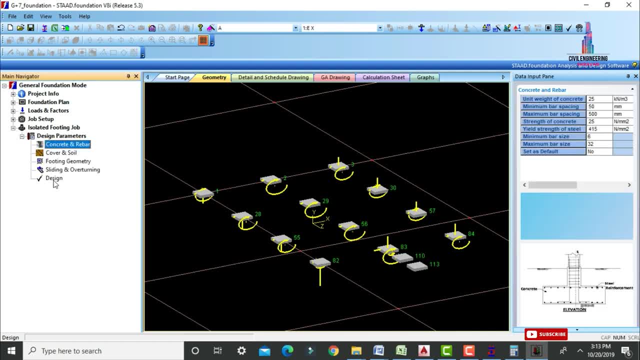 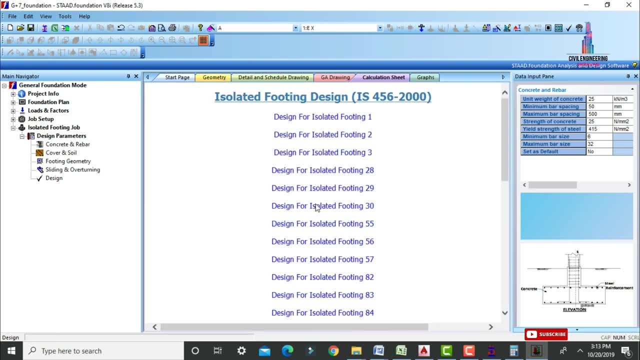 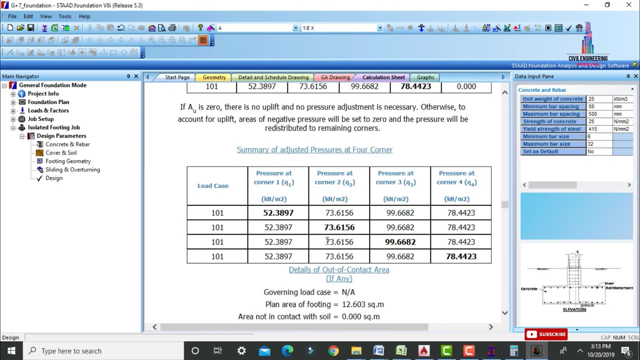 design and parameters. so click on design option, click on s button so it will design the isolated footing as per is456 2000 code. so this is the isolated footing design, so select isolated. So this is the each and individual calculation sheet and each and individual part for this. 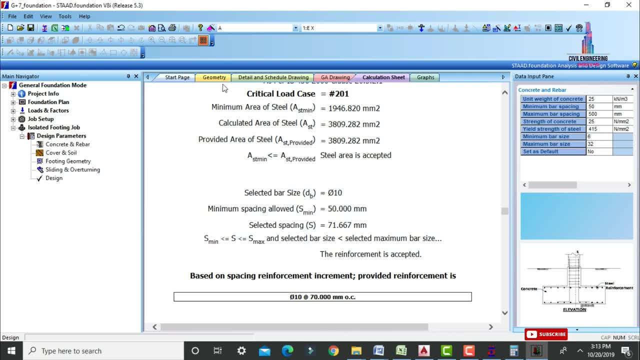 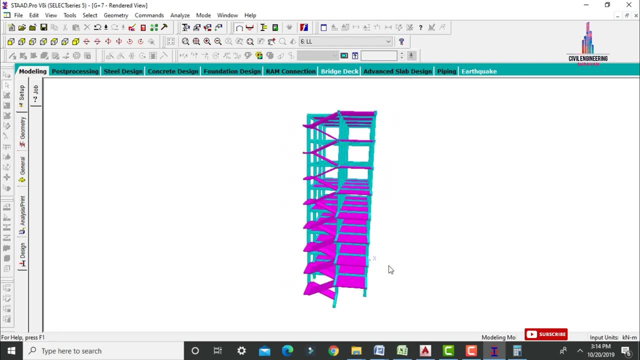 respected foundation design. So this is a starting page. geometry: click on details and drawing drawing calculation sheet. So this is the process analysis and designing of G plus seven storey building in high seismic zoning condition by using STAND PRO V8A software. Thank you.